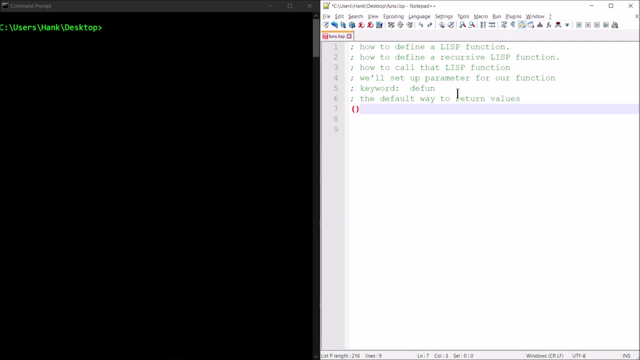 when we define the function, we're going to have an opening and closing parentheses. I like to split them up on different lines, because it feels a little bit more like C style blocks to me that way. Okay, so start off the function definition with the keyword defun. Then you have the name for your function, which in this case I'll call it add them, And so I'll add two numbers together, And so we've got a little bit more. 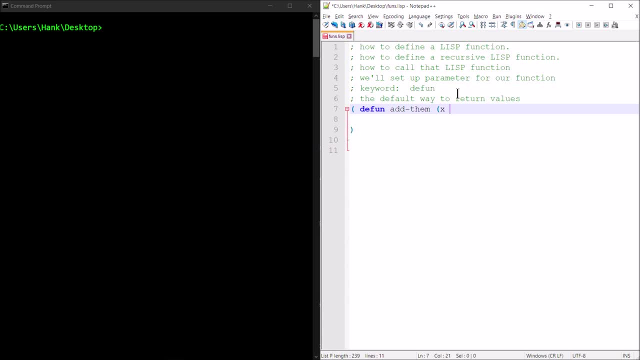 to make it interesting, We'll add three. We're going to have three parameters then, right, So I'll call those parameters X, Y and Z. Okay, now on the next line, what I'll do is I'll have my expression for performing the addition X, Y and Z. right, And I'm done. right, So what? What do you mean? you're done. Well, there's no explicit return statement necessary here, right? So by 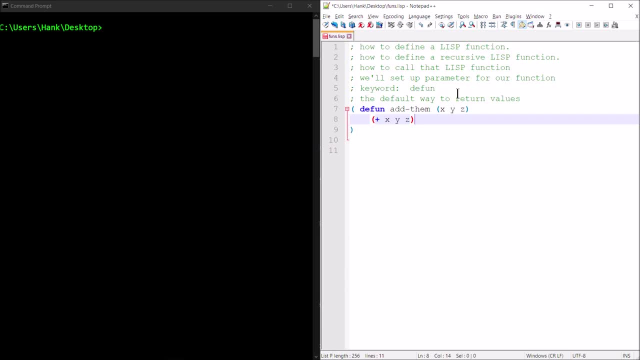 default. the way Lisp functions return values is they just return the last expression that was evaluated. Okay, so let's call this function and, you know, display the results on the screen. So I'll use a print statement to do that And we're going to call the function like you call anything else in Lisp. right? Put the name of the function, followed by some arguments, right, And let's go ahead. 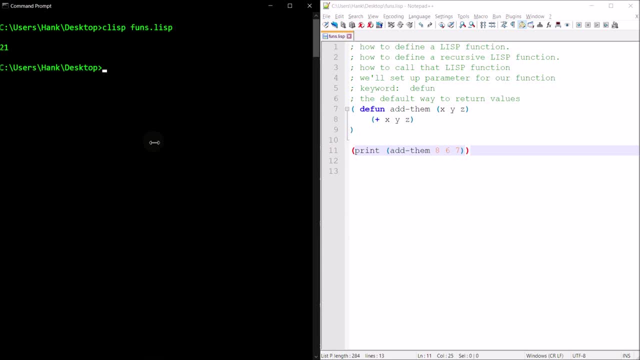 and run this and see what happens. right, So 21.. So 8 plus 6 is 14, plus 7 is 21.. Okay, then let's do another example here. How about we write a function that is going to find: 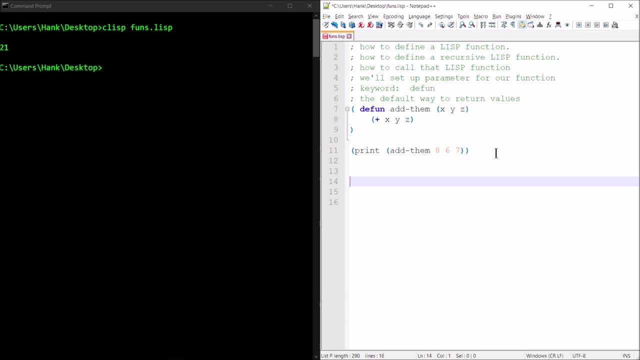 an average right. So that's usually a common thing to do here. So if we're going to do that, we'll do the defund thing And then we'll have a function called abg And we'll find the average of three numbers. 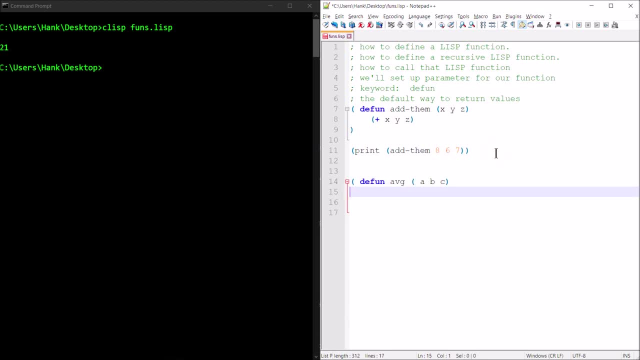 say abc, right, And so what's going to happen? so we're kind of an idea. the last expression evaluated is going to be the one that is returned, right? So I'm going to want to add those three numbers together, right? But then I need to divide those by three. 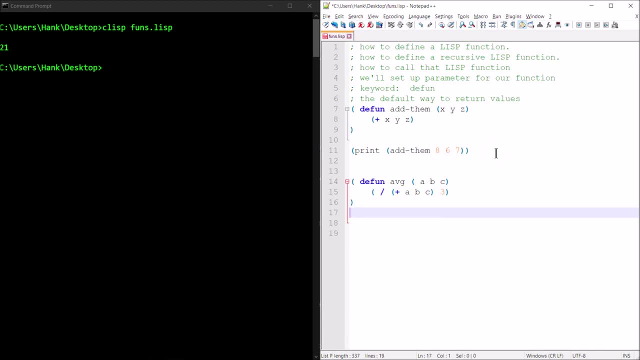 Okay, and so that's all. That's all that I need inside the function definition. So let's go ahead and call the function, And this time we'll set the value that's returned. we'll go ahead and put that into a, into a variable ands. Okay, so, abg, and we'll say 867.. Okay, and then I'll print out the average. 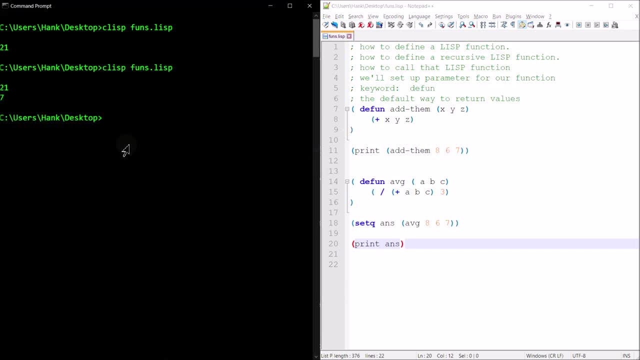 Okay, so let's see what happens. So average is 21 or 7.. 21 divided by three is seven. Okay, so next example: let's try to make a function that can return the bigger of two values. Okay, so let's do that. Now remember: last value evaluated is the one that's going to get returned. 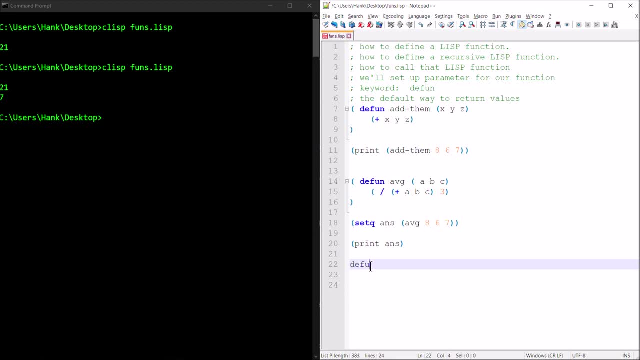 Right. So let's go ahead and define the function. Oops, Define. I'll call this bigger And we'll have a primer list of x and y. Okay, so I'm going to need to have myself an if statement, All right. so we'll say, if bigger x, y, then we'll go ahead and evaluate to one value. 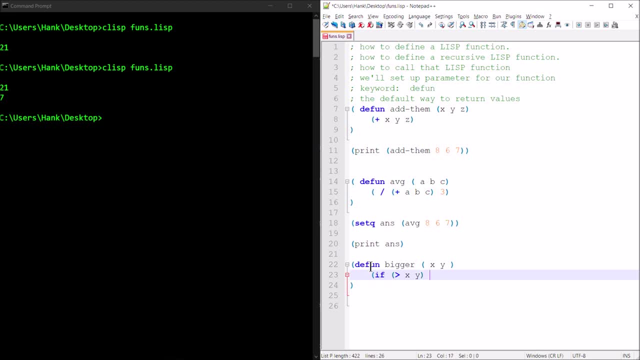 Otherwise we'll evaluate to another. So here's the thing, though Right, It has to evaluate an expression. So what I'll do is is I'll add x and 0 together, Right, To have that evaluation happen. So that way I'll have something returned. 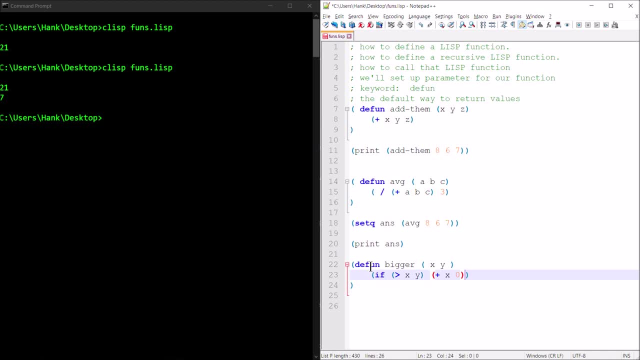 Right Now, remember, with if statements you can have an if else to where, if the thing is true, you know, if x is greater than y, then we'll execute this immediate statement right here, this immediate expression right here, Otherwise we can. 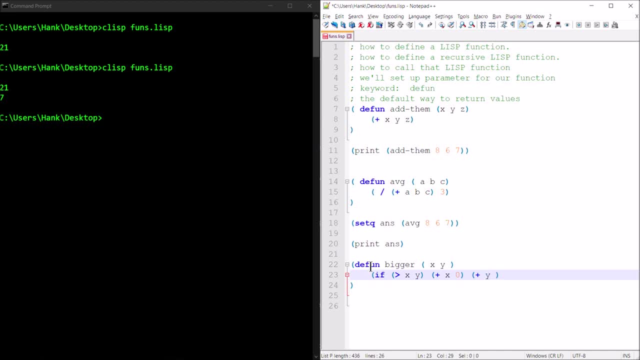 um, evaluate another one, right? So in this case we'll add y and 0 together. So if this is going to be true, right here, then we'll get this out, which will just be x, because x plus 0 is x. 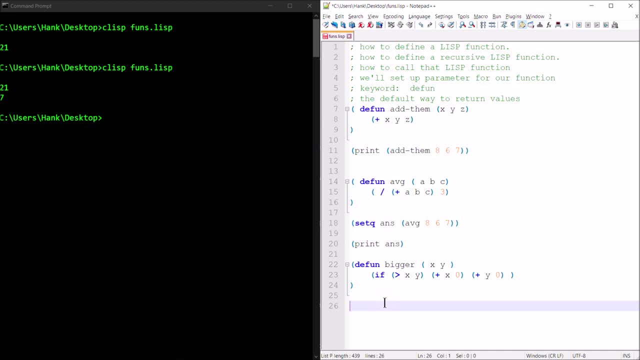 Or we'll get this one out right here. So let's go ahead and give that a try and see what happens. Um, so I'll just print it straight away. So print bigger: um 3, 9.. Right, So I should see what 9 on the screen. 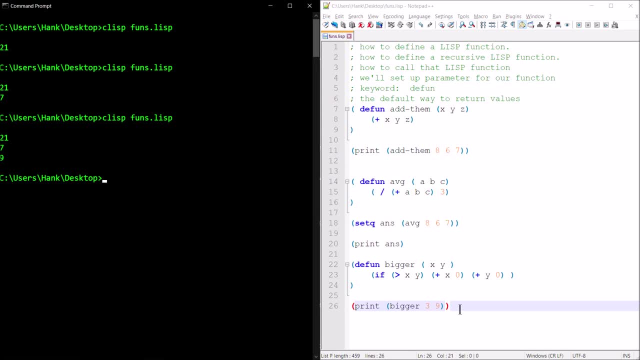 So let's try it Right? So there's your 9.. Um, cool, So let's try another one here. We'll go ahead and we'll give a shot at something recursive. Um, so, in addition to recursion, how about we do something with lists too? 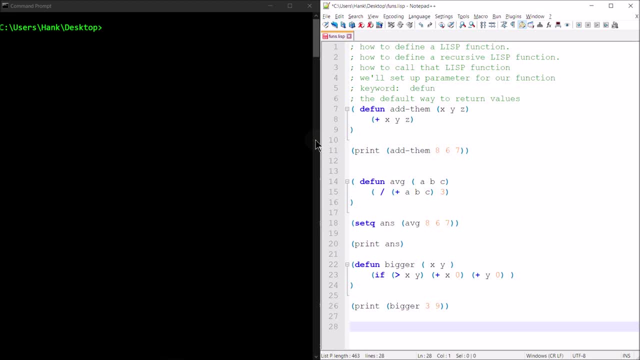 So we'll combine the two, We'll, we'll, uh, do something recursive with lists And uh, how about we? we print the lists backwards. We'll print one list backwards, right? So, in order to do that, 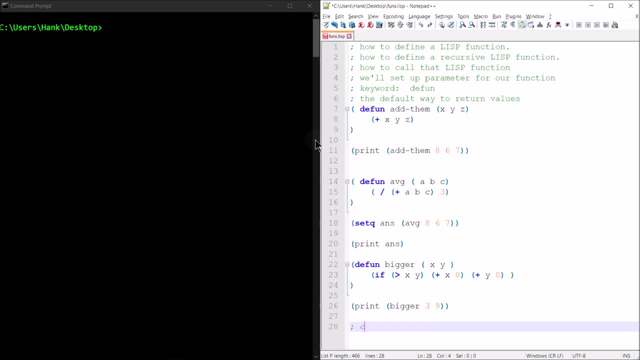 um, we're going to need just where we work with lists. Let's bring car in here. Let's bring cutter in here. Let's also bring in the null predicate. That's going to help us out with our base case, because we can't print anything if the list is empty. 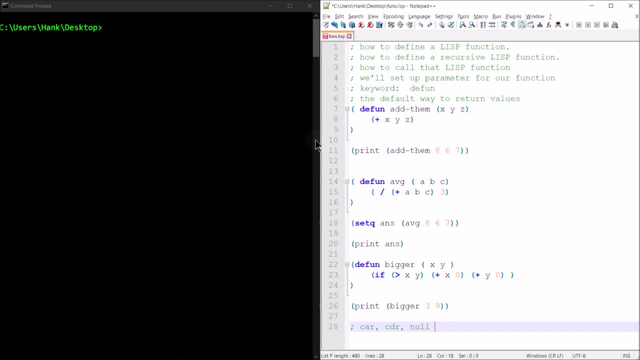 right, That'll end our recursion. when we no longer have anything left in the list, Then we'll bring in the logical operator here. So the idea is basically going to be like this: Uh, our base case is going to be an empty list. 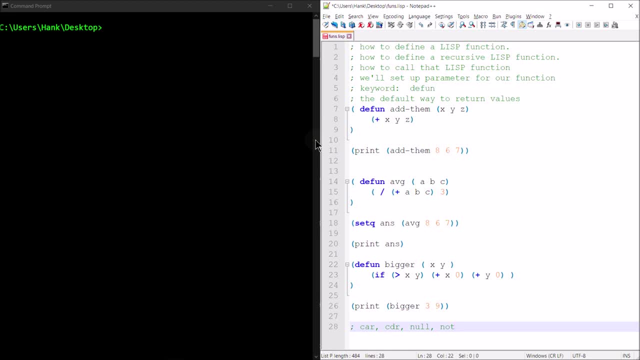 So the list is empty, We're done, Okay, But if it's not, then what we'll do is is we'll print the rest of the list and then we'll print the beginning of the list, the first time in the list, Right? 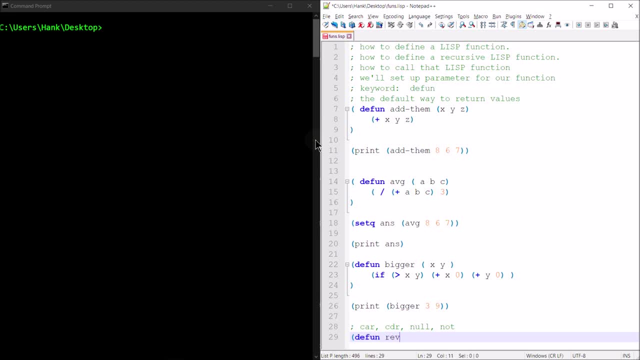 So let's, let's do it. So we'll call this function: uh, rev, list. have a single parameter, because one list, Okay, now here's the thing. Um, I'm going to need, I'm going to need to use two if statements to make this thing work. 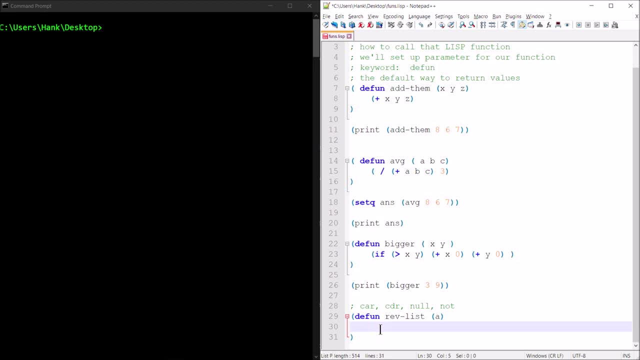 right, Um, two if statements, So let me throw them in here. We're going to say: if what right, If something, then something, Um, so what's the something? So, if not, no, not know what, if not, in all, a right. 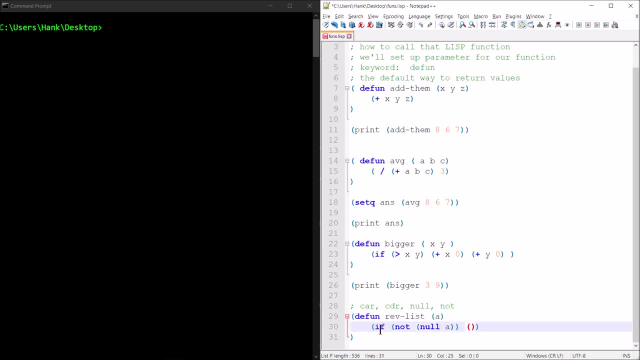 So if the list we passed is not null, then what are we gonna do? We're going to call ourselves. we're going to recursively print ourselves backwards. But what are we going to print? We're going to pass. we're going to pass the rest of the list. 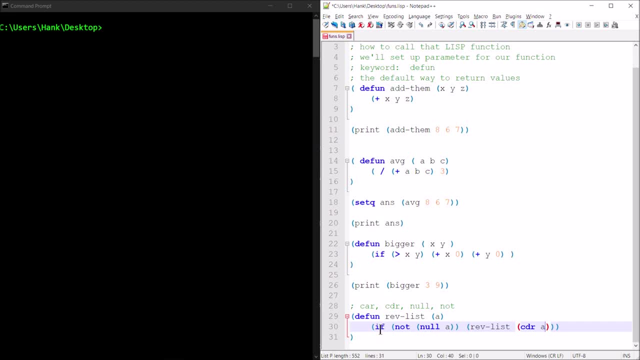 So that's where cutter comes in. Okay, so if the list is not null, first print the rest of the list, you know, recursively in reverse order. But if that's not true then we'll go ahead and check to see again. if we're not, don't have a empty list. 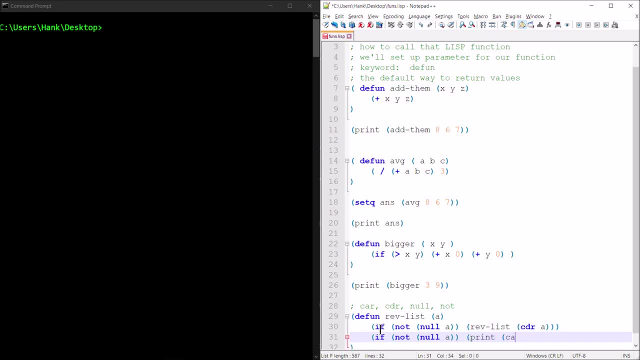 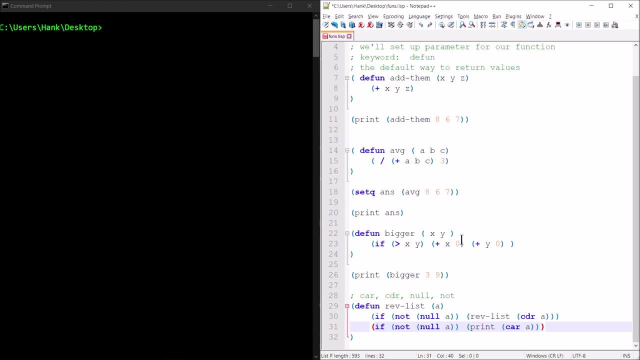 If we don't, then we'll go ahead and print what we'll print: the first item in the list. Okay, so that should be the end of our uh function, right? So I've got to do this for both lines here. 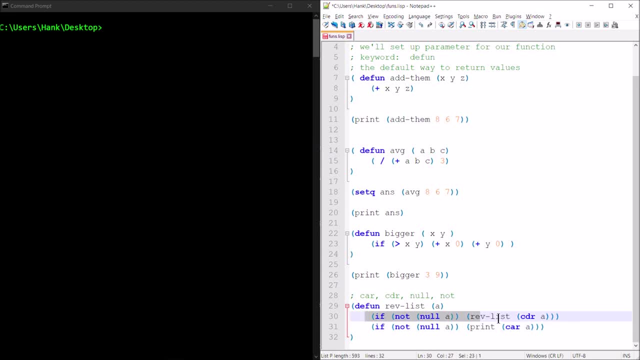 Um, I mean, we can write it a different way to make a little bit cleaner, but um, you know we're gonna go and do it this way, So if not, no, I go ahead and recursively do what we're going to do to ourselves, to the rest of the list. 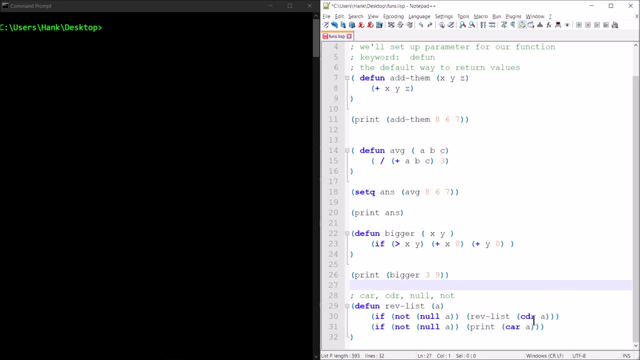 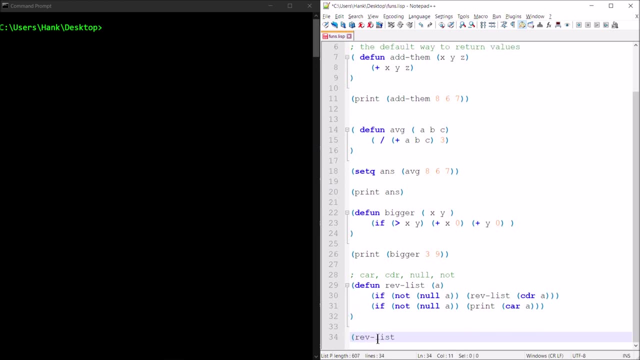 And if not, no lay after that. print the first time in the list. Okay, so let's go ahead and try it. Call it, And I'll just pass it a list. A, B, C, D, E, F. 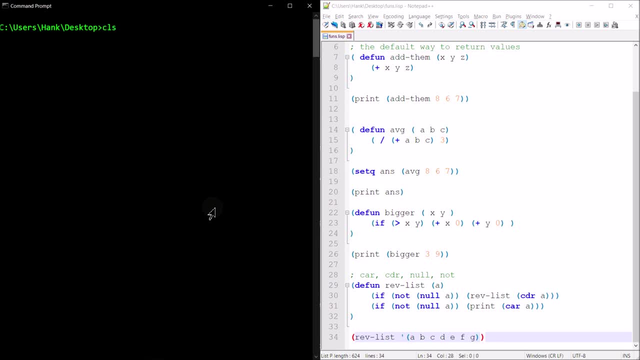 G, And let's try it, Okay. so there you go, right. So there's the G, there's the F, there's the E, there's the D, there's the C, there's the B, the there's the A. 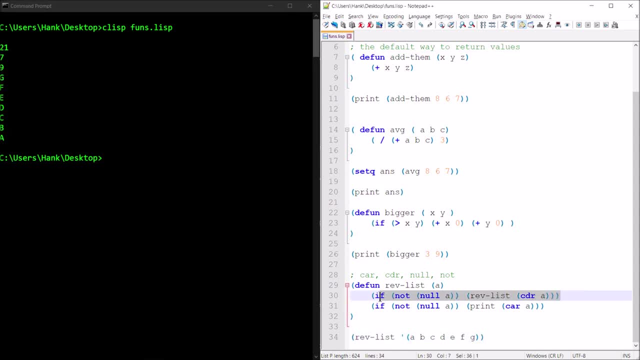 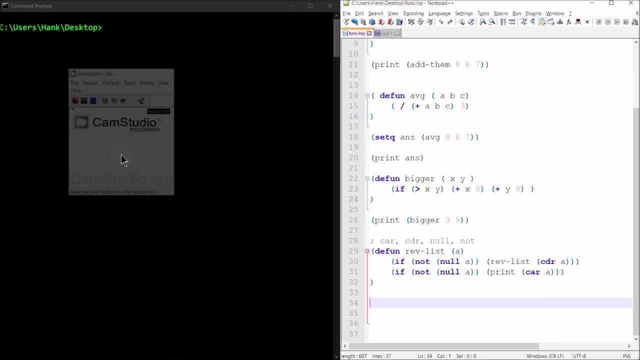 right, So it's in reverse order, because why we printed out the rest of the list and then we printed out the first item in the list? Okay, so one last example here. Um, how is something a little bit more complex? Uh. 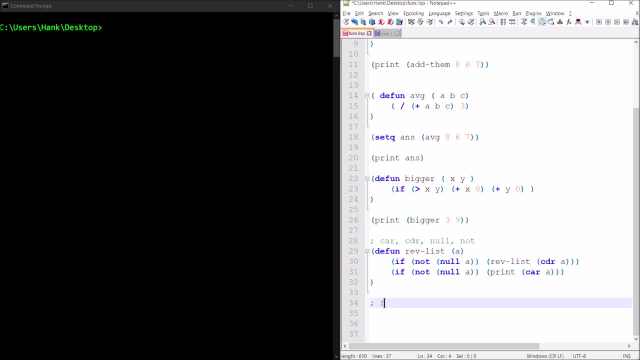 how about we? um, how about a function that counts the number of lists in a list, no matter how deeply nested they are, right? So what I mean by that is: let's say that I've got, um, I'll create a list here. 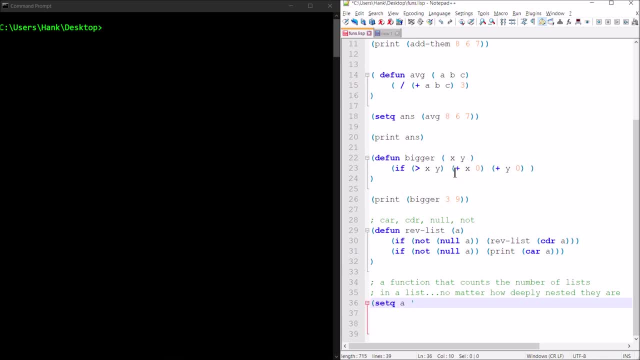 uh set Q A and I'll just make some stuff up here: A, B, C, D, E, F, G, H, I, J, K, L, right. So this would be zero right. 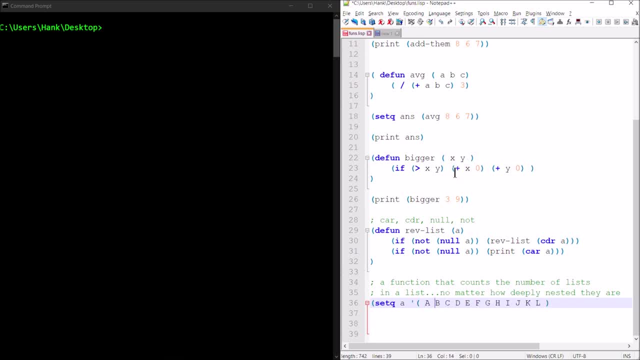 Because there's no lists inside this list, right. But if suddenly I put, you know, parentheses around D, E, F, G, well then there's one list in there, right. And if I put another one around I and J? 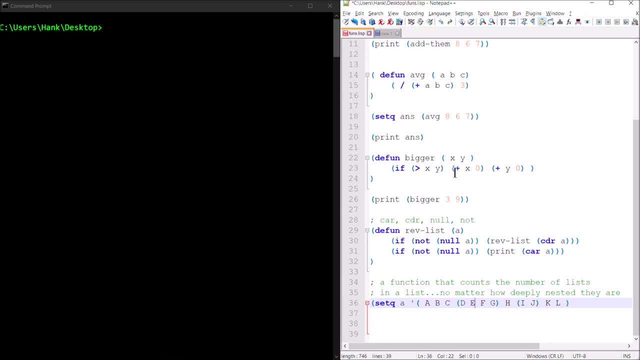 well then there's two lists in there, So my function should return two. Now what if I put um a list in between the E and the F? Well then there's now suddenly this: this: this outer list here contains: 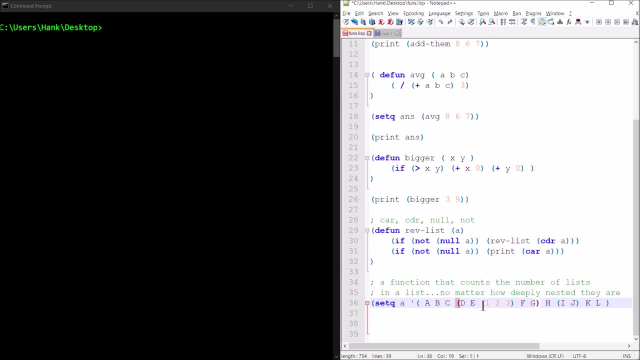 you know um, one list for that, two lists for that, three lists for that, right, Um. and then what if I add uh, one more in here? So um about GG, okay, So if I do that, 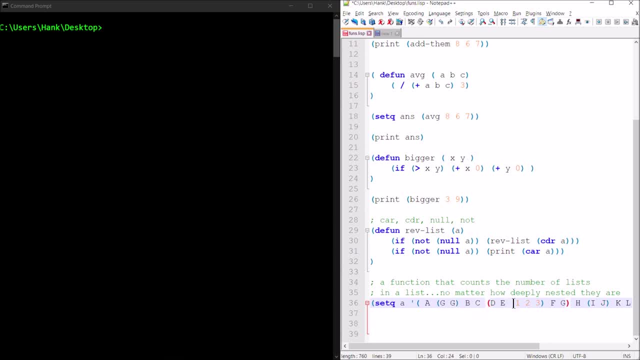 then I should have what a total of one, two, three, four, five lists in there, right? So how about we um write a function that's gonna count how many items are in that list? So uh, 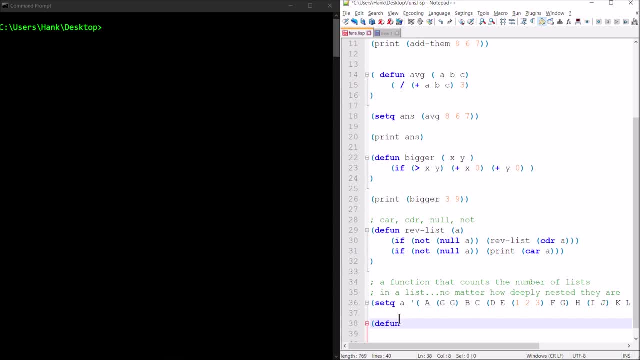 it's gonna have to be recursive. That'd be the easiest thing to do here, So we'll call this um, count lists, Okay, And I'll need one uh parameter And uh if the list is empty. 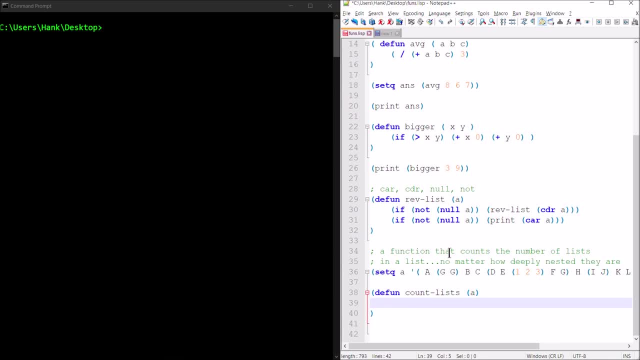 well then, obviously I shouldn't do anything, So I'm gonna use the COND decision structure here. Now, the difference between COND and IF is that COND is your. you know, you're used to the IF-ELSE-IF in C++. 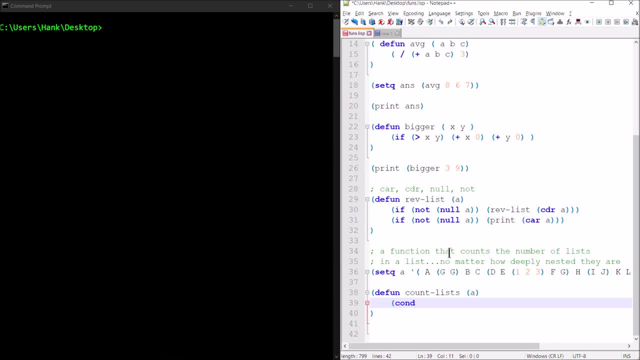 right, That's, that's what COND is. Um, basically, you're gonna have a series of test expressions And, um, if one of them is true, then the rest gets skipped. And, uh, if all of them are false. 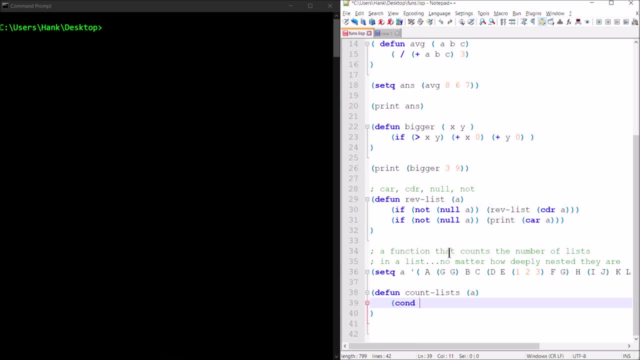 then you're gonna have a default option, right, So COND, And so the very first test I'm gonna have is gonna be if something is uh null, right, So if the list I passed this is null, well, 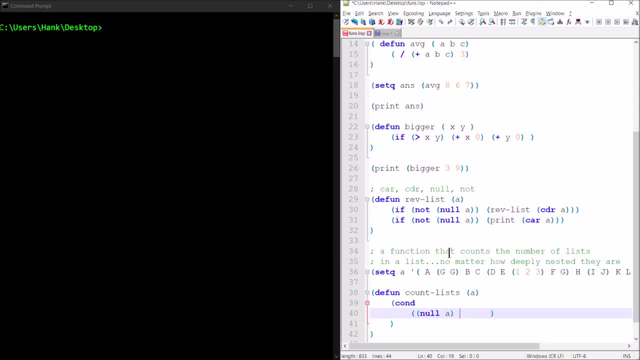 then there's nothing to do right. So that's gonna be my base case too. So once I've got an empty list, well, if the list itself is empty, well, there's no way that there can be a list in there. 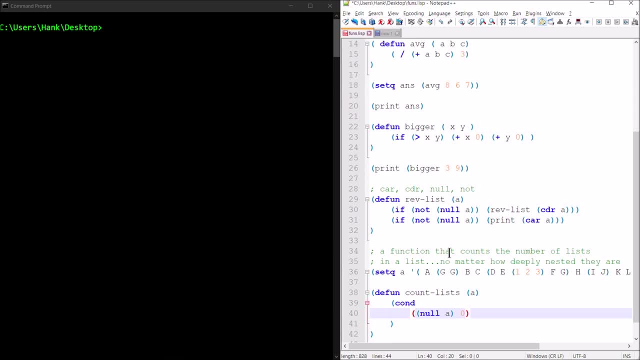 right. So naturally it would be, I'd be returning zero. Okay. But my second option is: you know what if instead, um, I've got a list right. What if what's been passed a is actually a list? 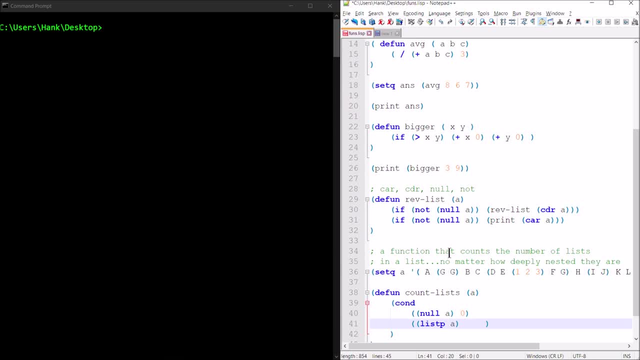 then, um, what I'll want to do is I'll want to check the um element, the first element of that list. So I'd want to grab, um, that very first element of it, Okay, And check to see if that's a list. 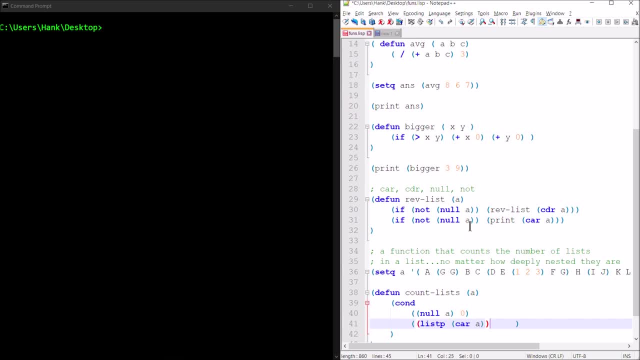 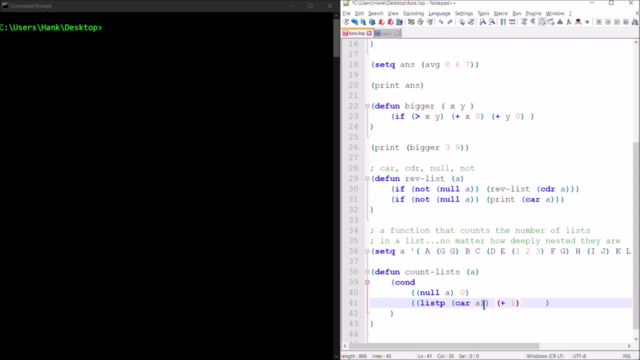 Now, if it is, then I need to count right. So I'm gonna add one, because that's a list that I have Um, um in my list that I'm counting, that I'm searching through right. So if the first element of the list that I passed to count lists is itself, 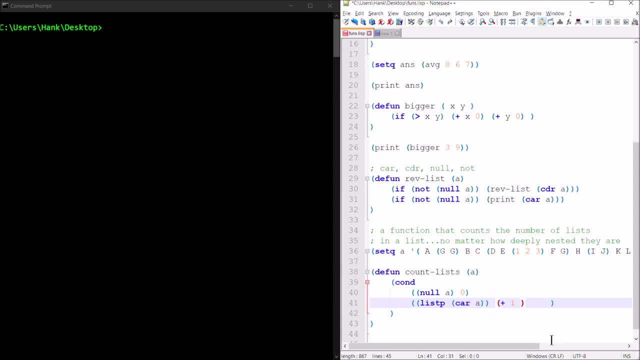 a list will plus one, right, But I'm not done yet because that would mean so. for example, I mean this would be a list right, So I'd be plus, wanting for that, but then I'd need to start searching the contents of that list for more. 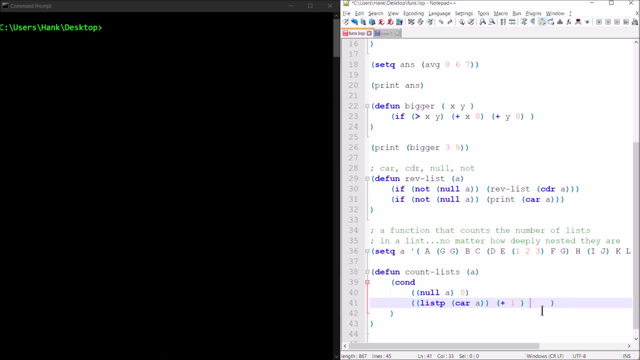 lists, right, So I will do that. So what I'll do is I'll say, all right, well then, let's go ahead and count lists in that list. Okay, So let me scroll over here a little bit. So I'm going to do that and make sure that my parentheses are all lined up. 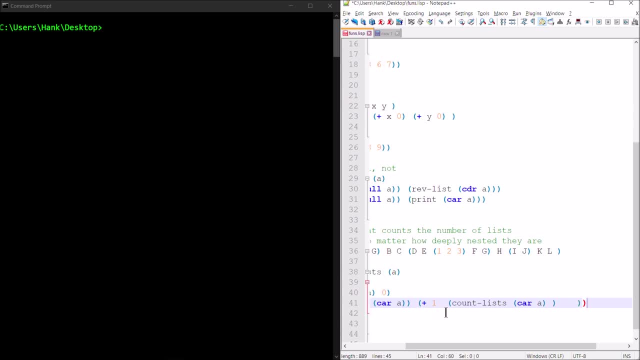 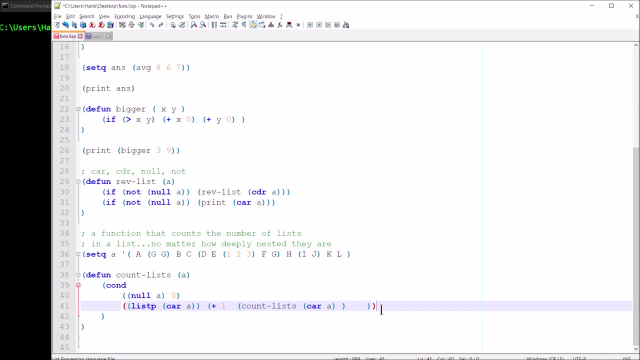 here. Okay Yeah, Let me make this just a little bit bigger here while we follow right This, Okay. So if let me just summarize again, cause it's a little complex here, cause it's recursive. So if the first element of list 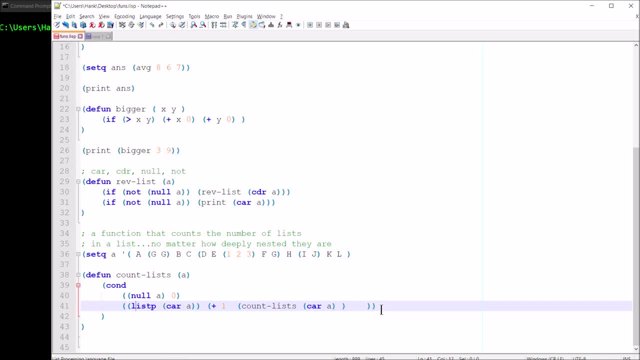 a, as specified by car a is itself a list that I'm going to add one right Plus account of how many lists are in that element, which is a list right. Whatever's in this list right here, I'm going to count how many lists are in there. 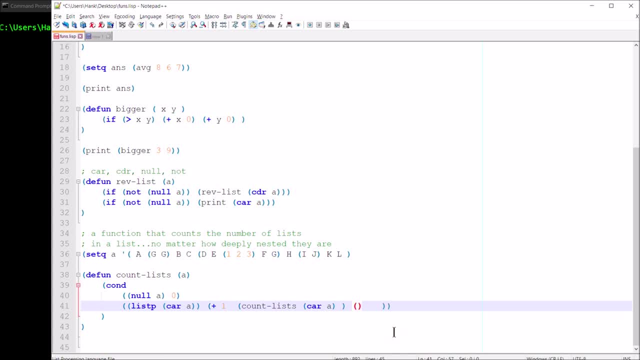 But in addition, I'm going to have to count everything that is remaining in a cutter. So now, if it's not a list, then I need to move on and count Zero, cause it's not a list, and continue looking through the rest of the. 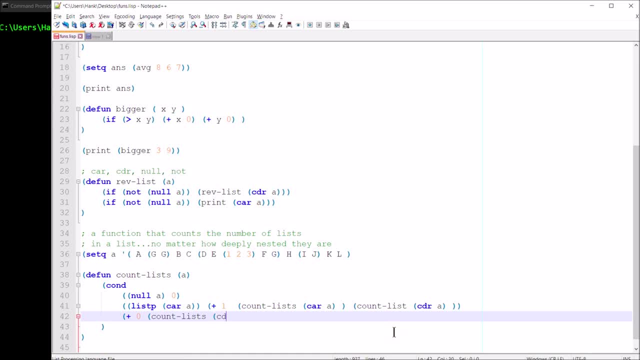 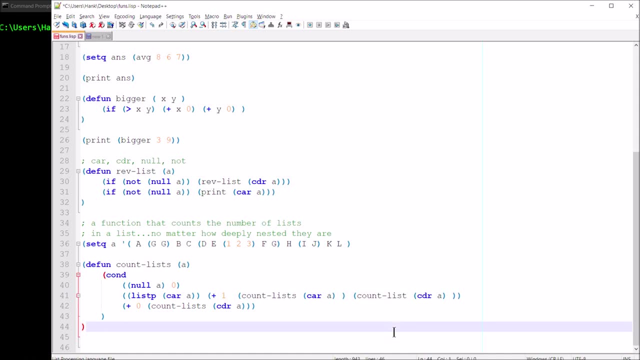 list. Okay, So something like that. So let me, let me, let me try to summarize it one more time, right Cause this, I know this is hard to follow, because recursive thinking always is, So let's see here. So I'm missing a closing part of the preface here. 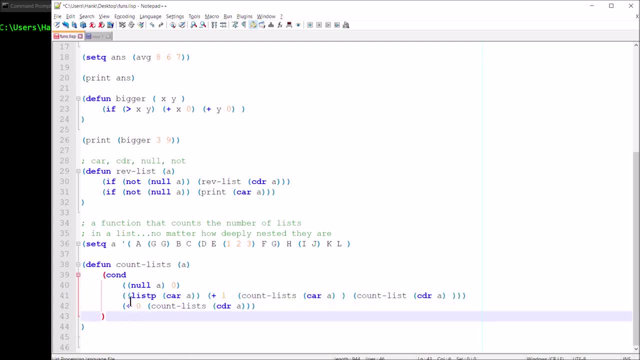 So let me get that and let me get that, Let me get that. Okay, So let's trace through this recursive function, right? So let's say that I'm going to call which I am. I'm going to call a count lists. 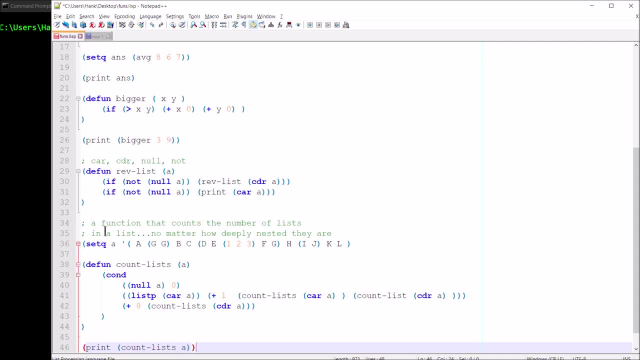 Okay, And I'm going to pass it this variable a. Okay, Now, when I first passed it, this entire list is going in, the whole thing, right? So is that an empty list? No, So then what's going to happen? 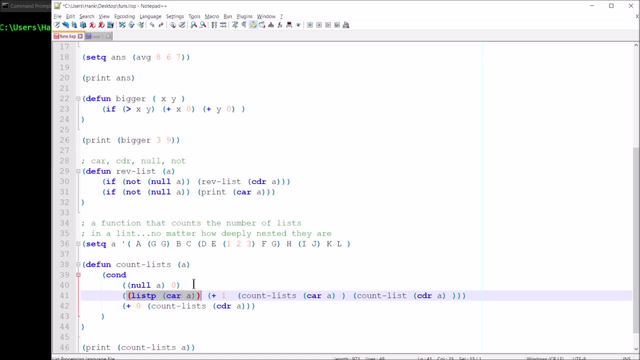 The second condition kicks in. Right, This test, right here. So car a is going to pull off the first element, which is a right there. Is that a list? No, So then we kicked down to here, And so then we add zero, plus we count the rest of the list. 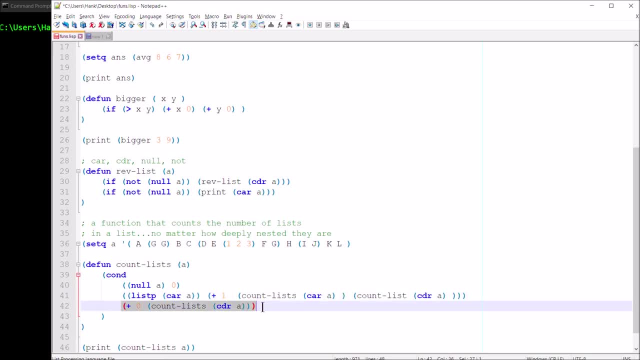 Right. So in the second instance of the function, right, This is going to be the remainder of the list, Right, And so then that gets past a in the second instance of the function, right. So here here, here here. 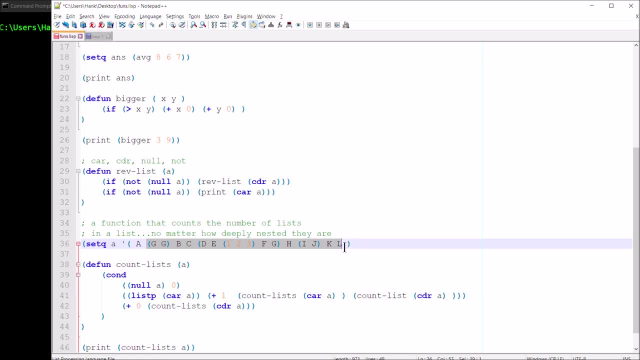 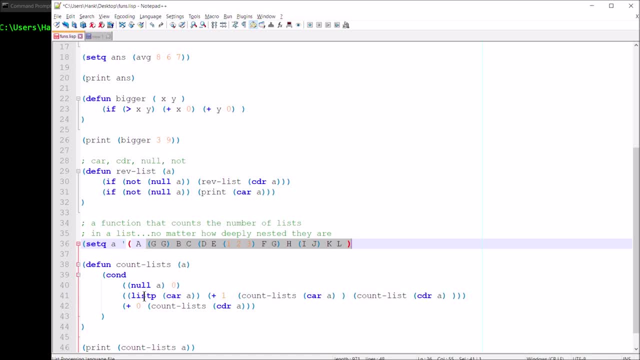 No. Now is the first element of the remainder. Is that a list? Yes, it is Right. So then what's going to happen is we're going to add one. now. this is where it gets kind of crazy, because we're going to add one for the gg. 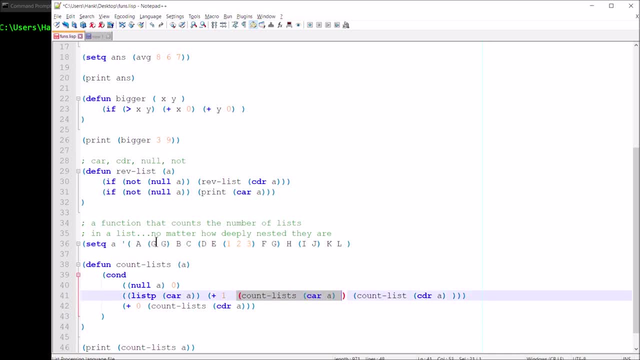 right, And so then we're going to call account list on the gg. That's going to start another instance of the function, Right? we're going to count list for the rest of the original list, right? So there's the two parts. 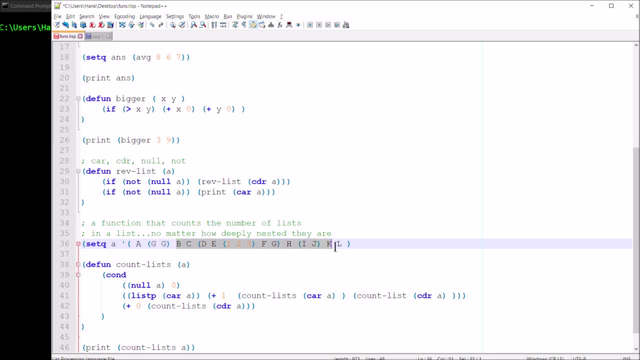 there's the GG, which is car of A in that case, and then here's the cutter of A right. So we're going to count lists on GG, which is car of A, then we're going to count lists on the cutter of. 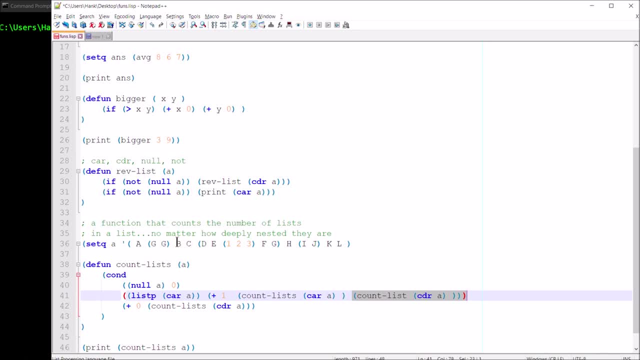 A, which is everything else right, And so it just keeps doing that over and over and over again. So for everything that's not a list, we add zero right, And as soon our base case is as soon as we hit a null list, which is to say a list that has nothing in it, then we're done right, Okay so 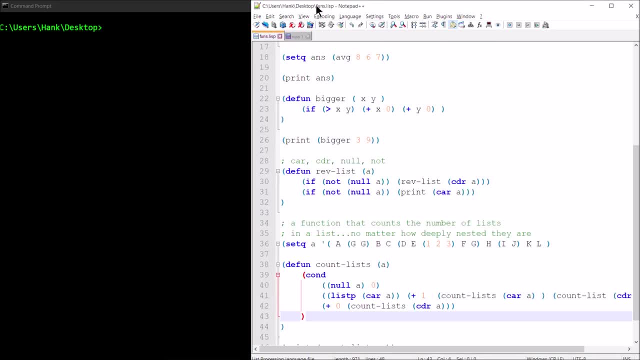 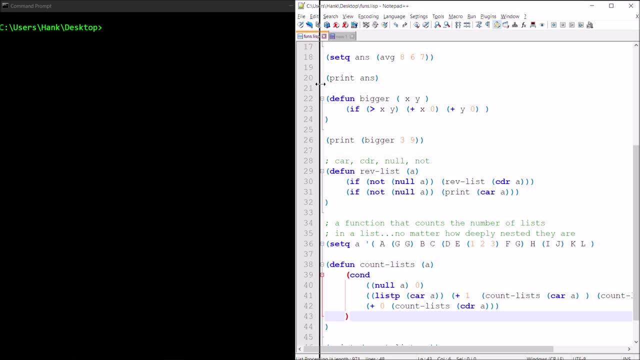 let's go ahead and try this. All right, so you got plenty of time to look at the code on your own. You know you can stop the video whenever you want to. You can try to work it out in your head. You can trace through it on your own just to see how that works. But let me go ahead and run it. 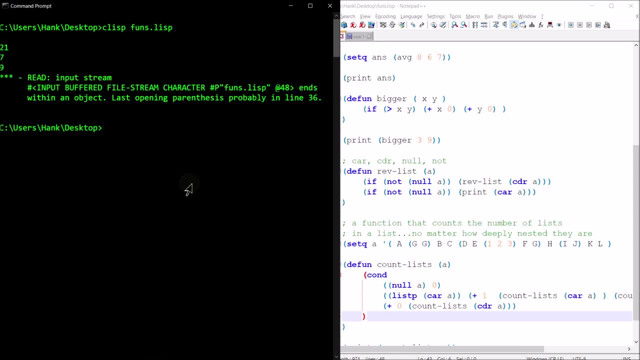 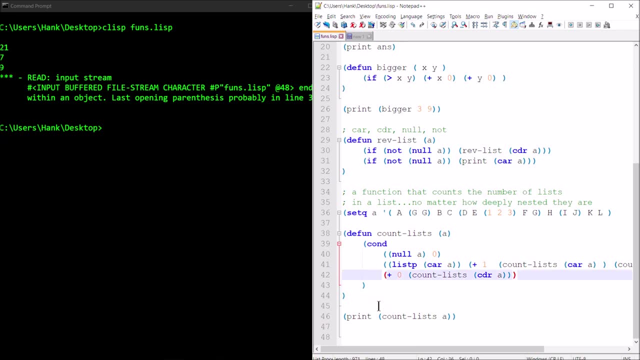 All right. so oh, I've got a parentheses somewhere. that shouldn't be, So let's go find our parentheses here. See our mismatched parentheses. Okay, it looks like probably way the heck up here on 936, right? So let's try one more time. 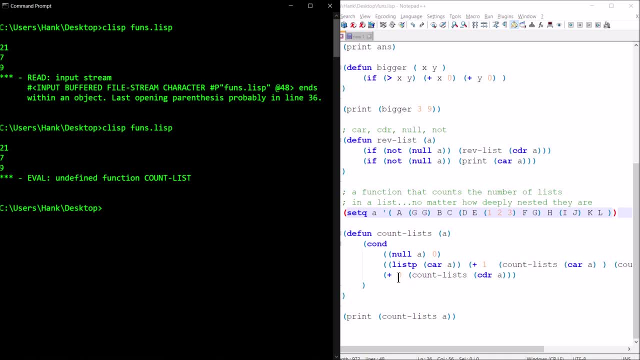 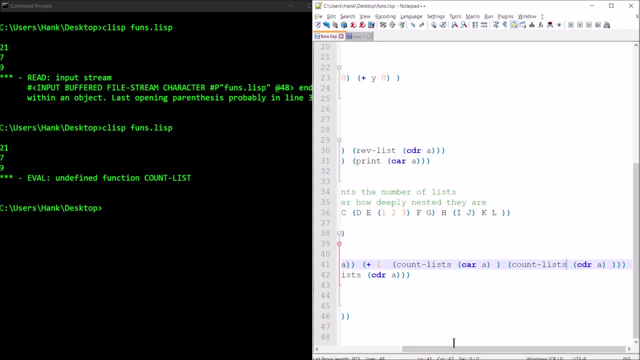 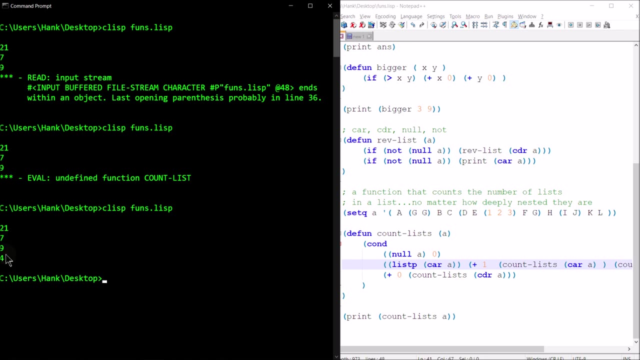 All right, so I got a 11. Count list, Okay. so, oh, forgot an S, So one more time. Okay, cool, So let's check. So it says four, right, So this is the result of this last call. 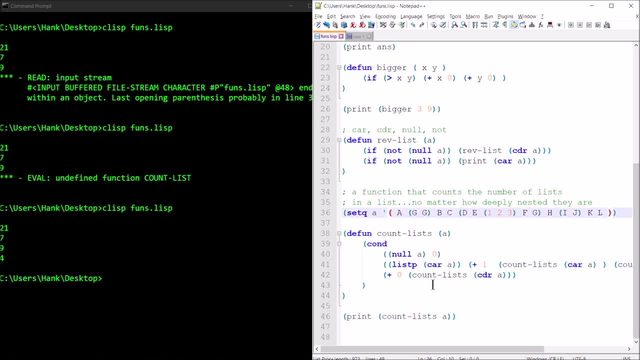 right here on line 46.. So, how many lists do we have inside of our list? Well, here's one right GG is a list. Here's two right G through G, But also one, two, three, So that's three. And then there's the IJ, So there's four.